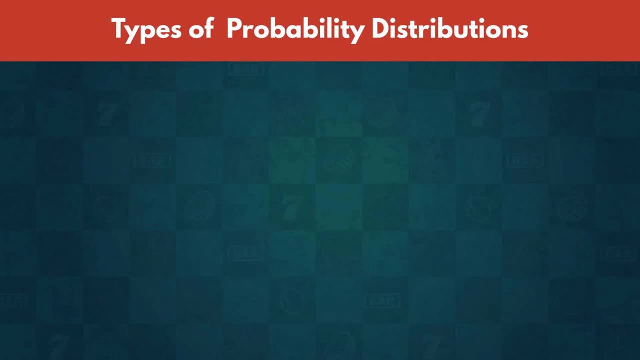 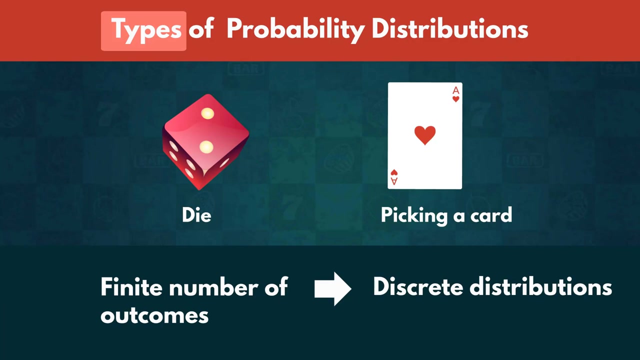 and what kind of events they can be used to describe. Certain distributions share features, so we group them into types. Some, like rolling a die or picking a card, have a finite number of outcomes. They follow discrete distributions. Others, like recording time and distance in track and field, have infinitely many outcomes. 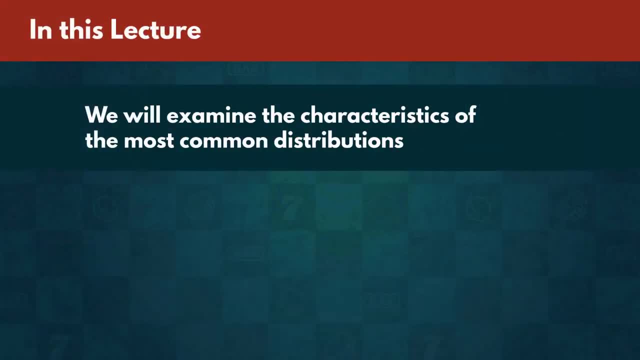 They follow continuous distributions. We are going to examine the characteristics of some of the most common distributions. For each one, we will focus on an important aspect of it or when it is used. Before we get into the specifics, you will need to know the proper notation we implement when defining distributions. 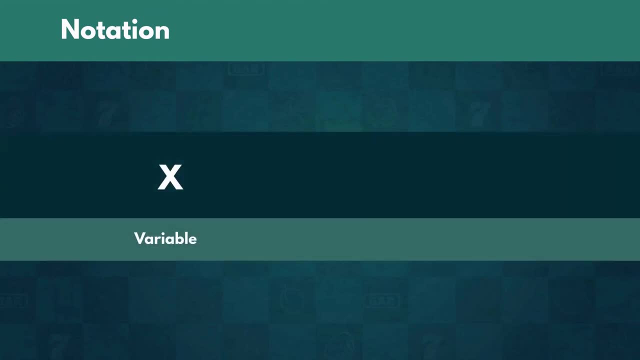 We start off by writing down the variable name for our set of values, followed by the tilde sign. This is superseded by a capital letter depicting the type of the distribution and some characteristics of the dataset, in parentheses. The characteristics are usually mean and variance. 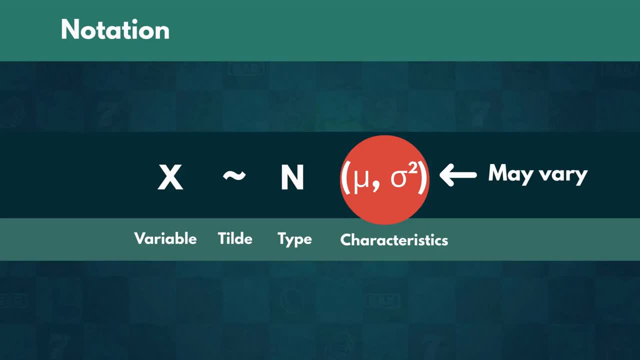 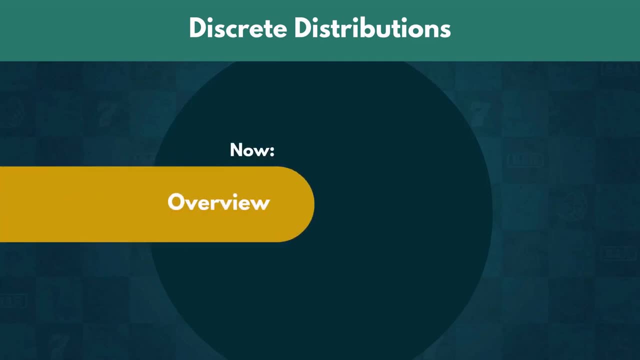 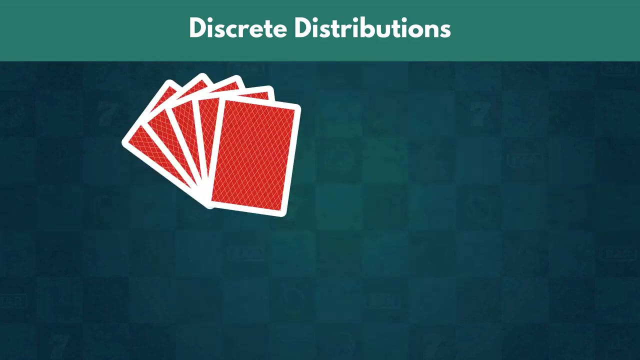 but they may vary depending on the type of the distribution. Alright, Let us start by talking about the discrete ones. We will give an overview of them and then we will devote a separate lecture to each one. So we looked at problems relating to drawing cards from a deck or flipping a coin. 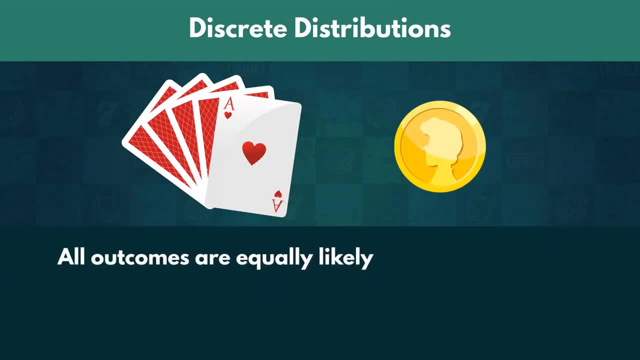 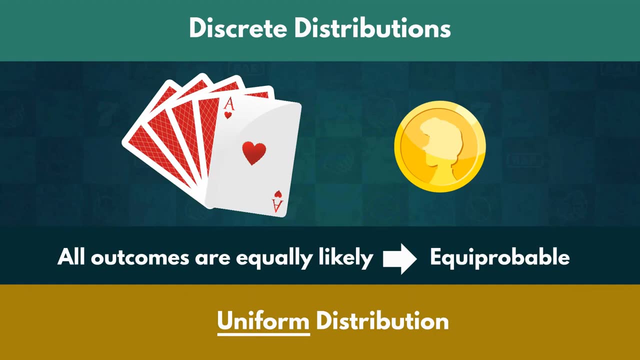 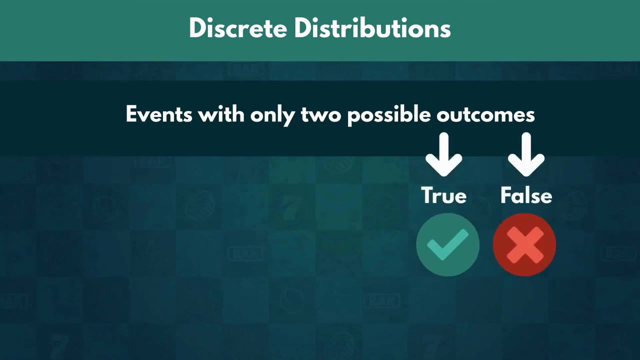 Both examples show events where all outcomes are equally likely. Such outcomes are called equiprobable, and these sorts of events follow a uniform distribution. Then there are events with only two possible outcomes: true or false. They follow a Bernoulli distribution. 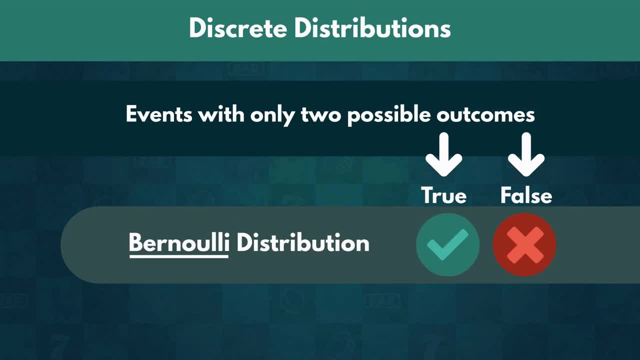 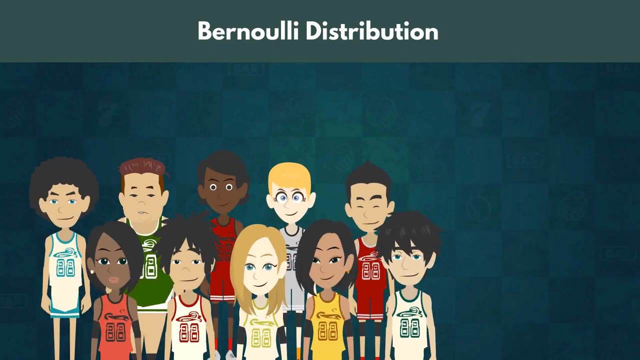 Regardless of whether one outcome is more likely to occur. any event with two outcomes can be transformed into a Bernoulli event. We simply assign one of them to be true and the other one to be false. Imagine we are required to elect a captain for our college sports team. 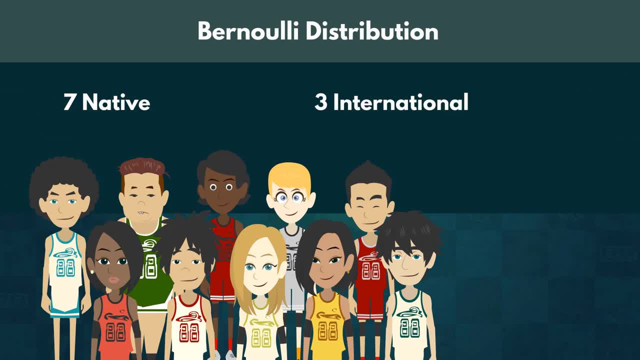 The team consists of seven native students and three international students. We assign the captain being domestic to be true and the captain being an international as false. Since the outcome can now only be true or false, we have a Bernoulli distribution. Now, if we carry out a similar experiment several times in a row, 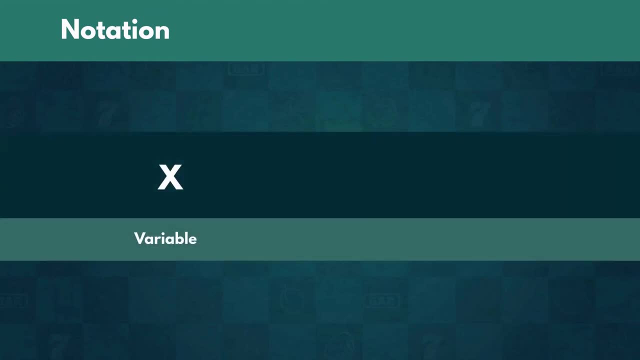 We start off by writing down the variable name for our set of values, followed by the tilde sign. This is superseded by a capital letter depicting the type of the distribution and some characteristics of the dataset, in parentheses. The characteristics are usually mean and variance. 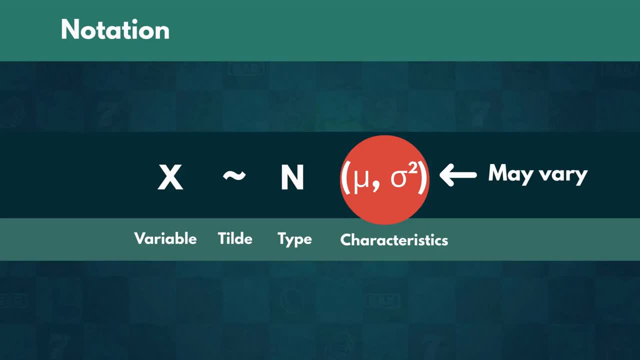 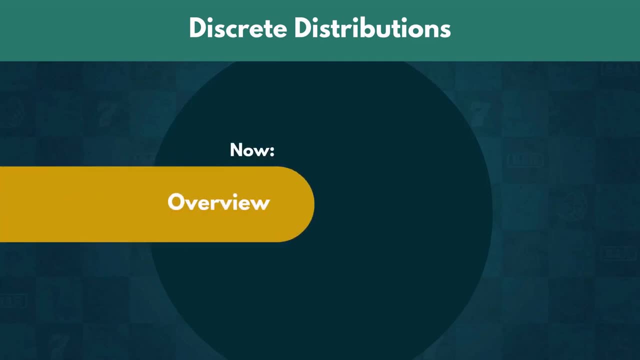 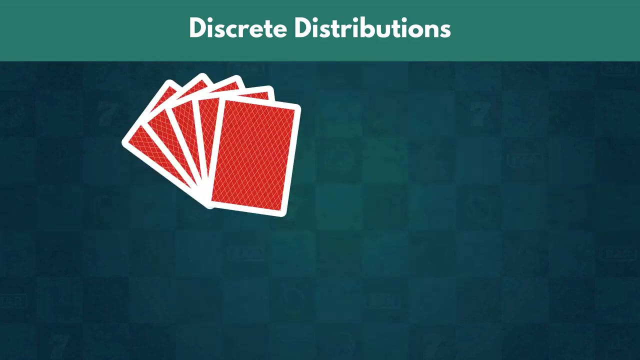 but they may vary depending on the type of the distribution. Alright, Let us start by talking about the discrete ones. We will give an overview of them and then we will devote a separate lecture to each one. So we looked at problems relating to drawing cards from a deck or flipping a coin. 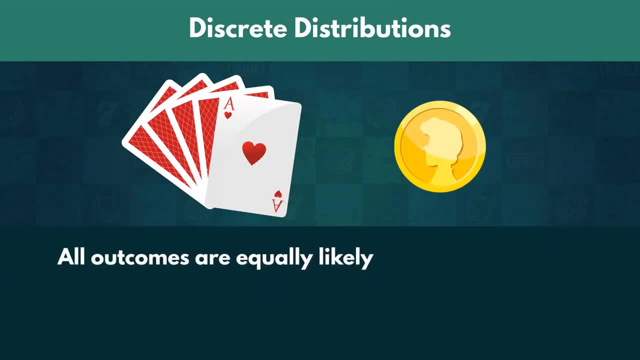 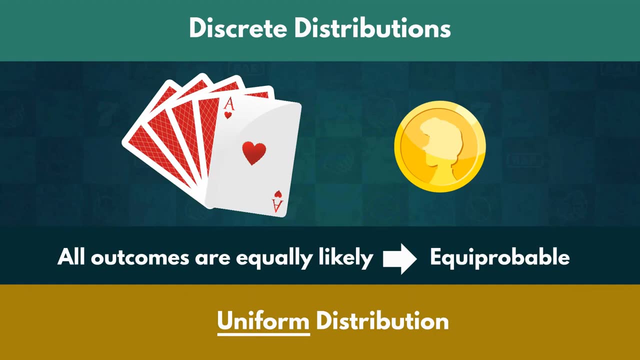 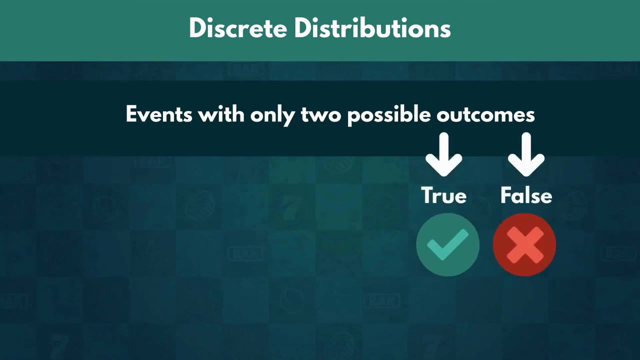 Both examples show events where all outcomes are equally likely. Such outcomes are called equiprobable, and these sorts of events follow a uniform distribution. Then there are events with only two possible outcomes: true or false. They follow a Bernoulli distribution. 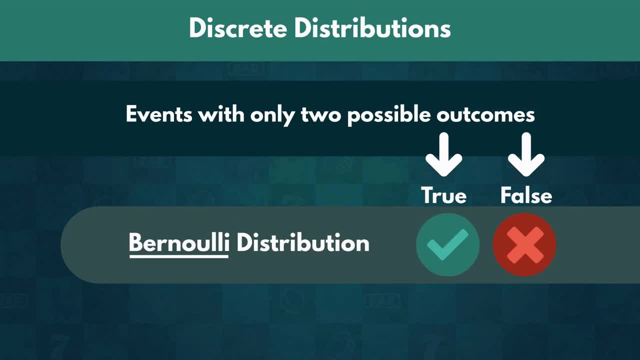 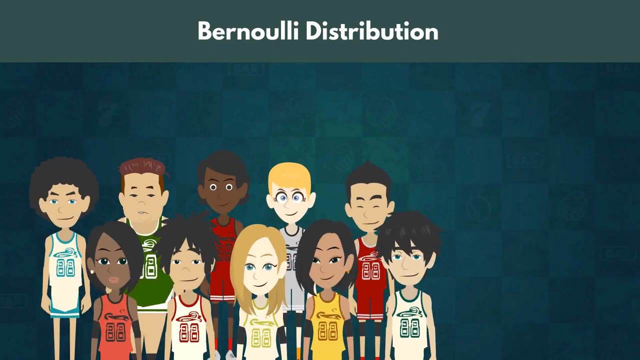 Regardless of whether one outcome is more likely to occur. any event with two outcomes can be transformed into a Bernoulli event. We simply assign one of them to be true and the other one to be false. Imagine we are required to elect a captain for our college sports team. 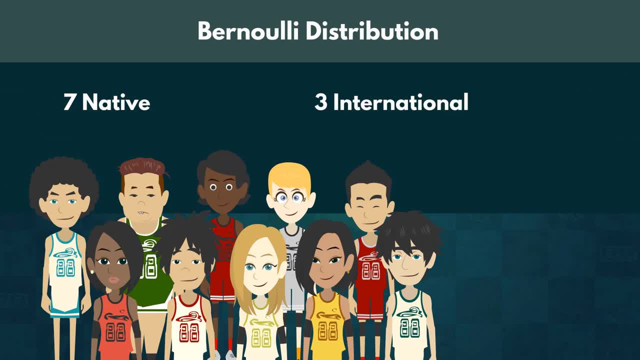 The team consists of seven native students and three international students. We assign the captain being domestic to be true and the captain being an international as false. Since the outcome can now only be true or false, we have a Bernoulli distribution. Now, if we carry out a similar experiment several times in a row, 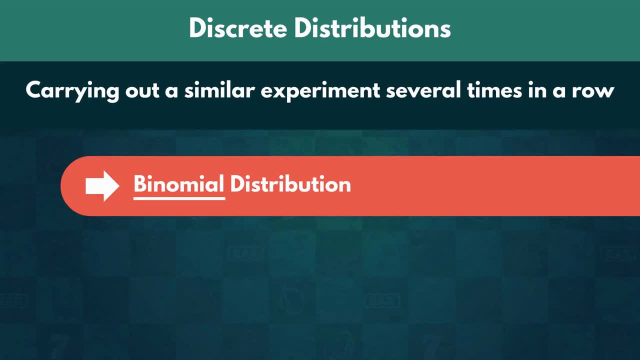 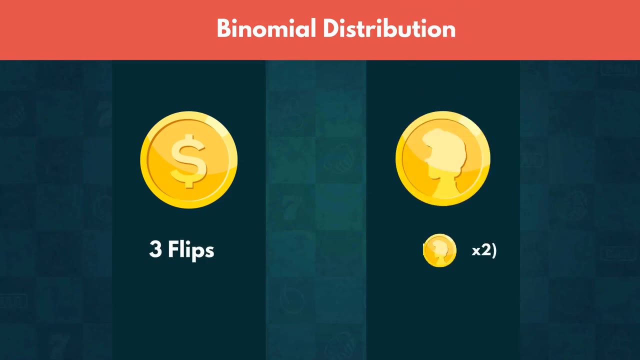 we are dealing with a binomial distribution, Just like the Bernoulli distribution. the outcomes for each iteration are two, but we have many iterations. For example, we could be flipping the coin we mentioned earlier three times and trying to calculate the likelihood of getting heads twice. 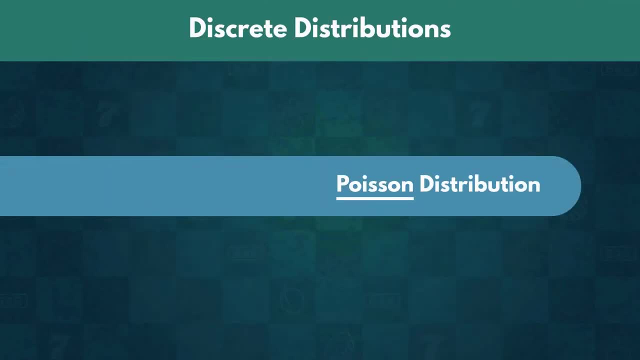 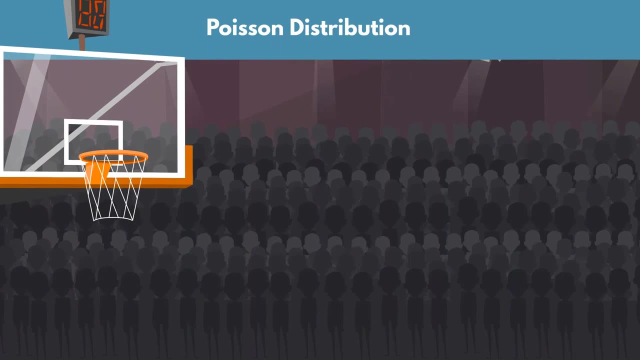 Lastly, we should mention the Poisson distribution. We used it when we want to test out how unusual an event frequency is for a given interval. For example, imagine we know that so far LeBron James has averaged 35 points per game during the regular season. 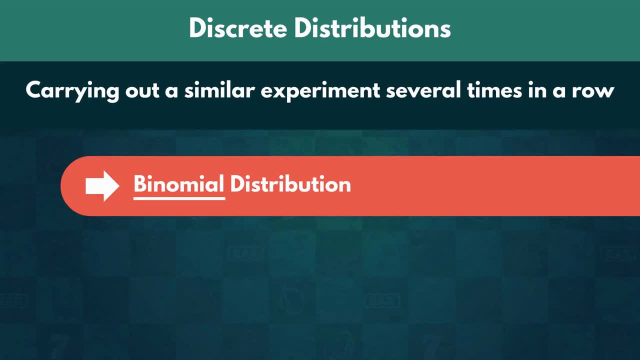 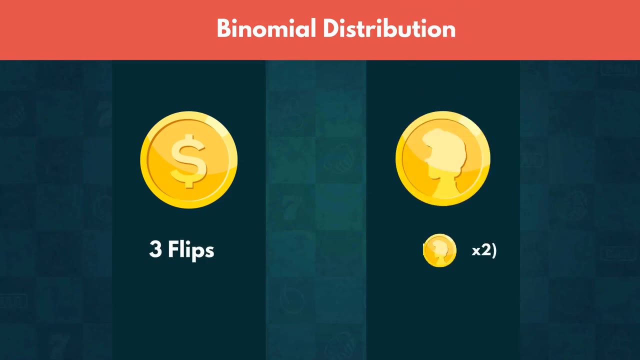 we are dealing with a binomial distribution, Just like the Bernoulli distribution. the outcomes for each iteration are two, but we have many iterations. For example, we could be flipping the coin we mentioned earlier three times and trying to calculate the likelihood of getting heads twice. 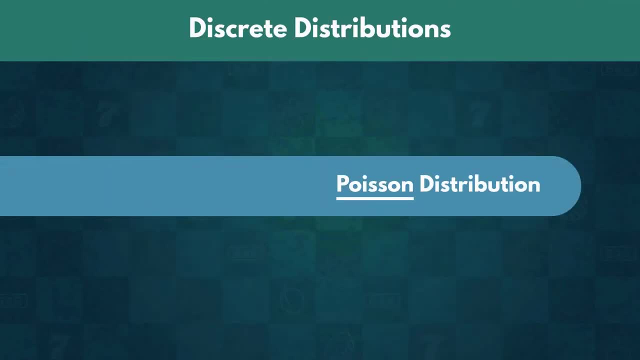 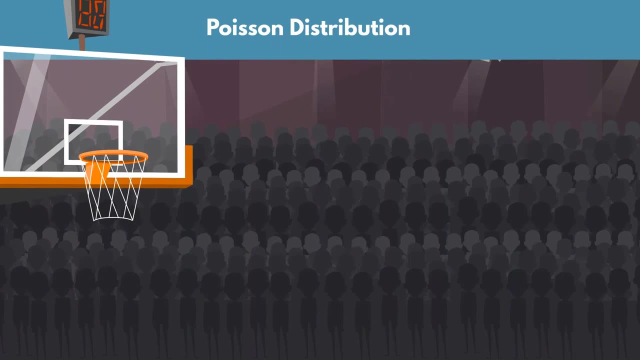 Lastly, we should mention the Poisson distribution. We used it when we want to test out how unusual an event frequency is for a given interval. For example, imagine we know that so far LeBron James has averaged 35 points per game during the regular season. 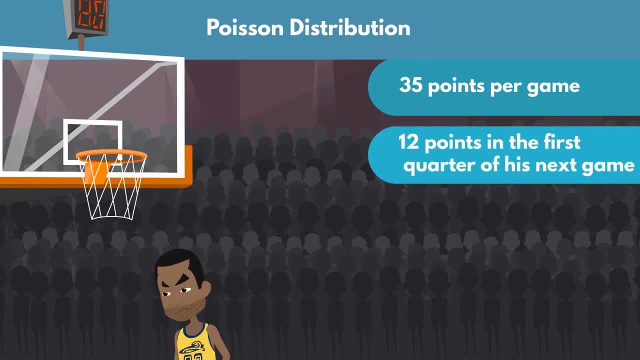 We want to know how likely it is that he will score 12 points in the first quarter of his next game. Since the frequency changes, so should our expectations for the outcome. Using the Poisson distribution, we are able to determine the chance of LeBron scoring exactly 12 points for the specified time interval. 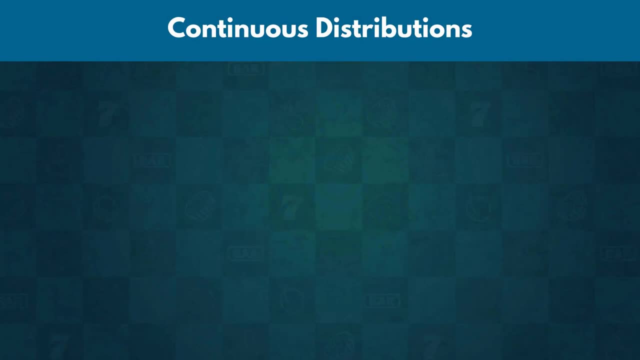 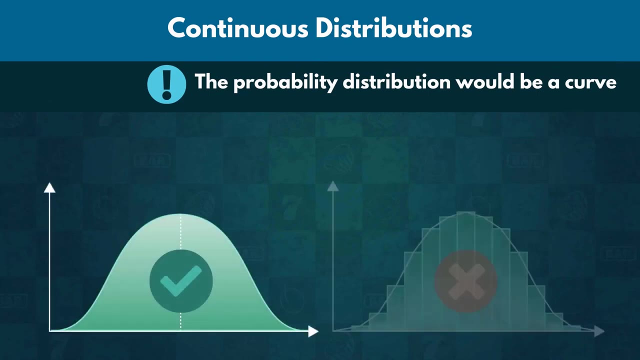 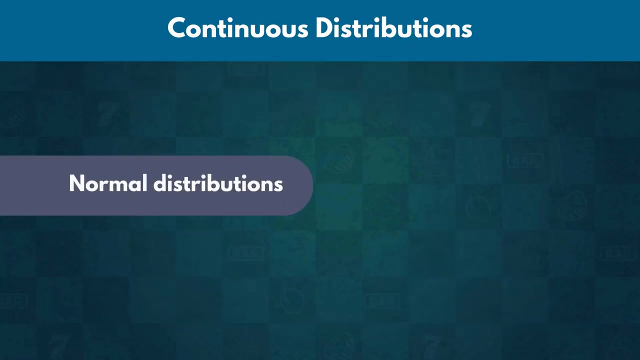 Great. now on to the continuous distributions. One thing to remember is that, since we are dealing with continuous outcomes, the probability distribution would be a curve, as opposed to unconnected individual bars. The first one we will talk about is the probability distribution. The outcomes of many events in nature closely resemble this distribution, hence the name normal. For instance, according to numerous reports throughout the last few decades, the weight of an adult male polar bear is usually around 500 kilograms. However, there have been records of individual species weighing anywhere between 350 kilograms and 700 kilograms. Extreme values like 350 and 500 kilograms are usually around 500 kilograms. 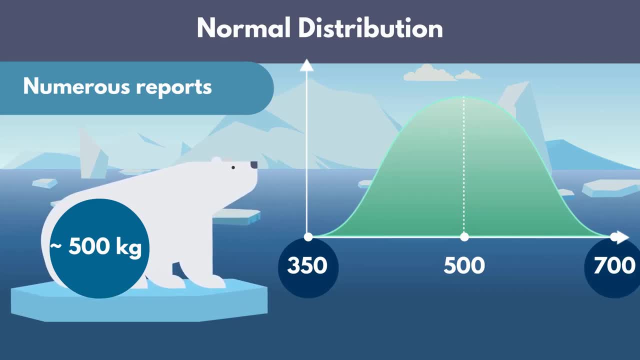 The average weight of an adult male polar bear is usually around 500 kilograms. The altitudes like 350 and 700, are called outliers and do not feature very frequently in normal distributions. Sometimes we have limited data for events that resemble a normal distribution. 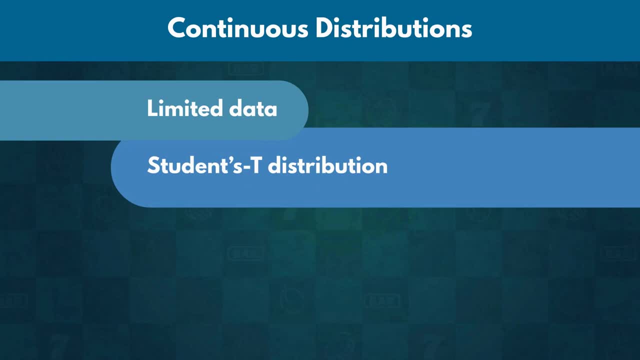 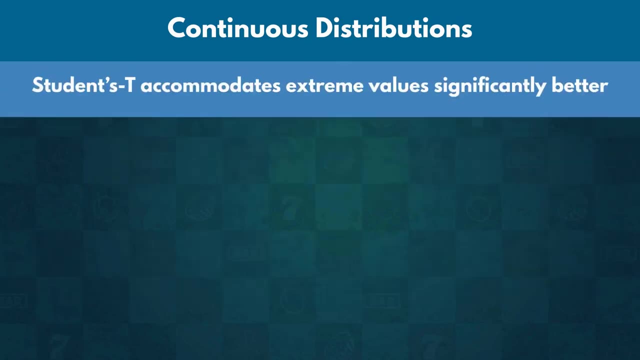 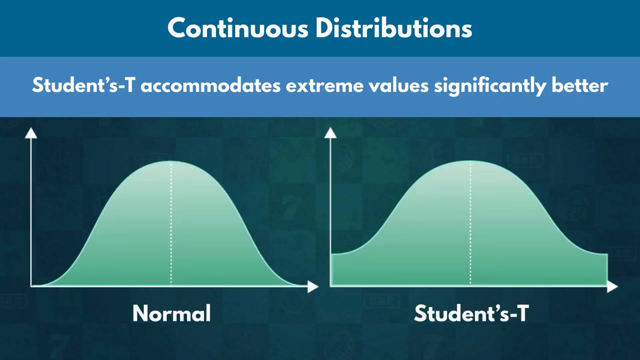 In those cases we observe the student's t distribution. It serves as a small sample approximation of a normal distribution. Another difference is that the students t accommodates extreme values significantly better. Graphically that is represented by the curve having fatter tails. 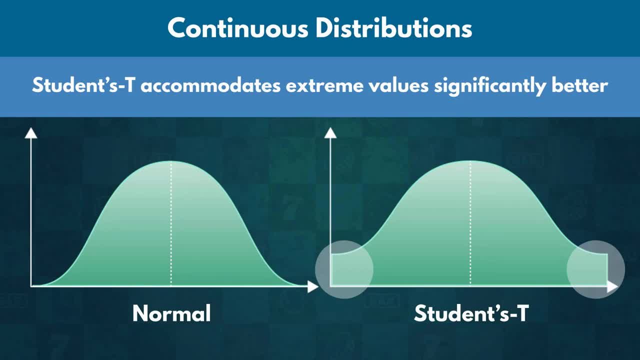 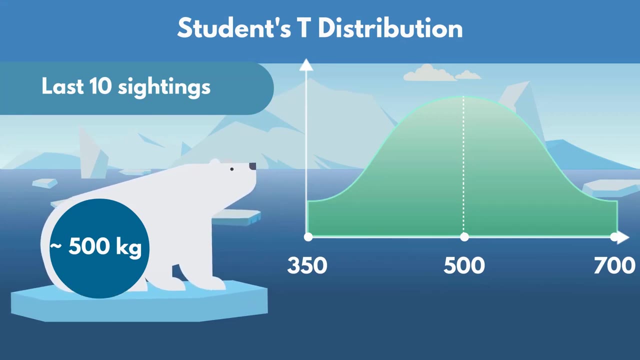 Overall, this results in a larger number of values located far away from the mean. so the curve would probably more closely resemble a student's t-distribution than a normal distribution. Now imagine only looking at the recorded weights of the last 10 sightings across Alaska. 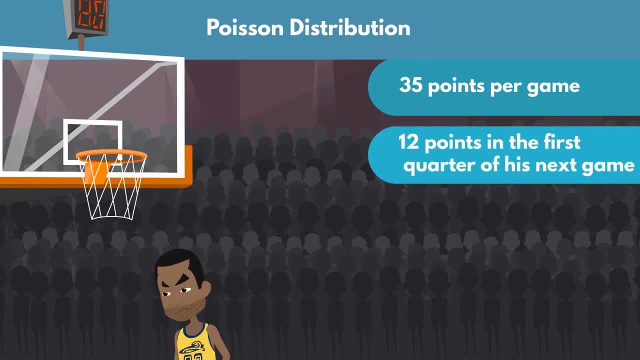 We want to know how likely it is that he will score 12 points in the first quarter of his next game. Since the frequency changes, so should our expectations for the outcome. Using the Poisson distribution, we are able to determine the chance of LeBron scoring exactly 12 points for the specified time interval. 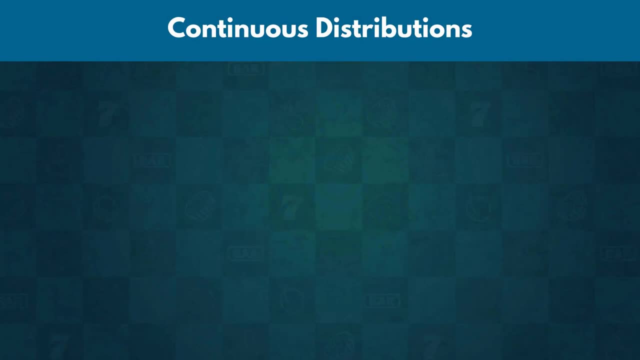 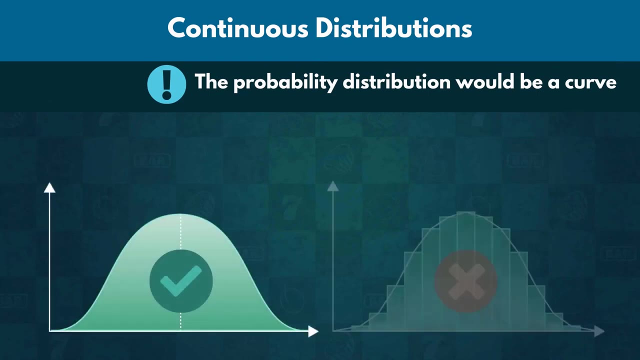 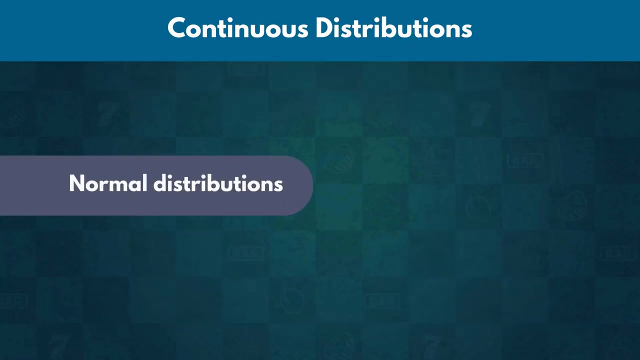 Great. now on to the continuous distributions. One thing to remember is that, since we are dealing with continuous outcomes, the probability distribution would be a curve, as opposed to unconnected individual bars. The first one we will talk about is the probability distribution. The outcomes of many events in nature closely resemble this distribution, hence the name normal. For instance, according to numerous reports throughout the last few decades, the weight of an adult male polar bear is usually around 500 kilograms. However, there have been records of individual species weighing anywhere between 350 kilograms and 700 kilograms. Extreme values like 350 and 500 kilograms are usually around 500 kilograms. The average weight of an adult male polar bear is usually around 500 kilograms. The other 다시llation of probability is that most individuals weighs over a thousand kilograms, and the average weight of an adult male polar bear is usually around 600 kilograms. The average weight of an average male polar bear is usually around 750 kilograms. 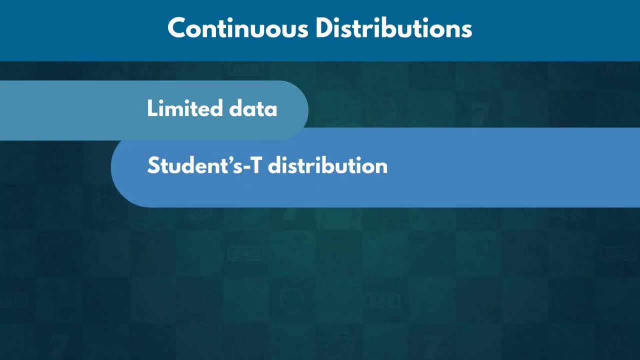 What we have noticed is that the squared-up number of many events, like 350 and 700, are called outliers and do not feature very frequently in normal distributions. Sometimes we have limited data for events that resemble a normal distribution. Sometimes we have limited data for events that resemble a normal distribution. 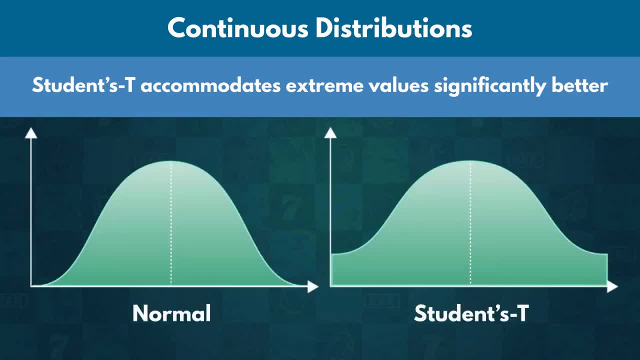 significantly better. Graphically. that is represented by the curve having fatter tails. Overall, this results in a larger number of values located far away from the mean. so the curve would probably more closely resemble a student's t-distribution than a normal. 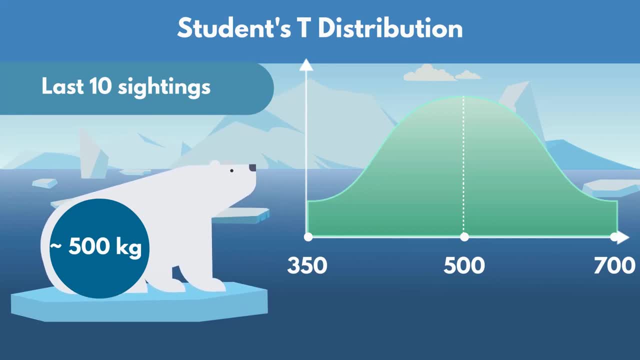 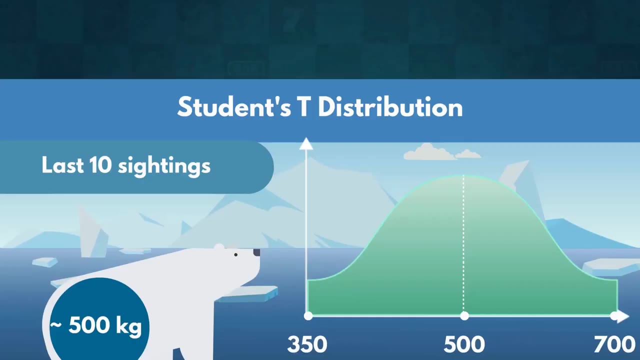 distribution. Now imagine only looking at the recorded weights of the last 10 sightings across Alaska and Canada. The lower number of elements would make the occurrence of any extreme value represent a much bigger part of the population than it should. Good job everyone. 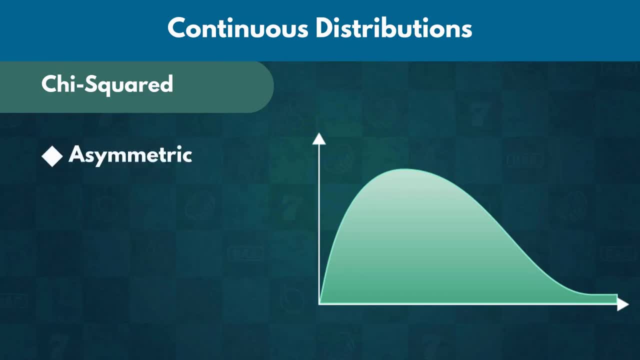 Another continuous distribution we would like to introduce is the Chi-squared distribution. It is the first asymmetric continuous distribution we are dealing with, as it only consists of non-negative values. Graphically, that means that the Chi-squared distribution always starts with a negative value. 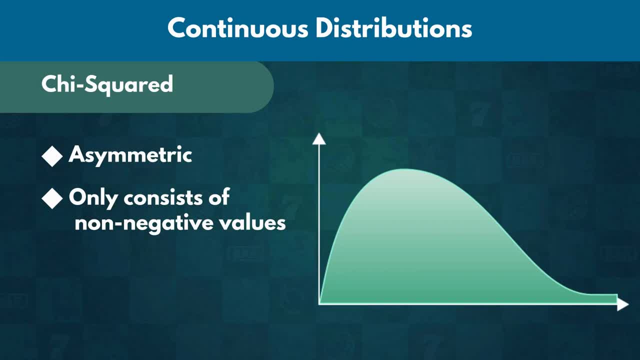 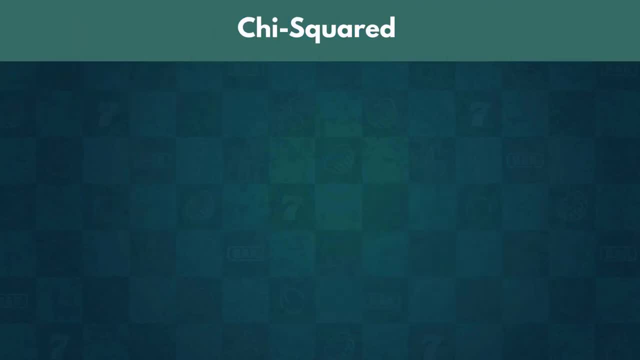 It starts from zero on the left. Depending on the average and maximum values within the set, the curve of the Chi-squared graph is typically skewed to the left. Unlike the previous two distributions, the Chi-squared does not often mirror real-life events.